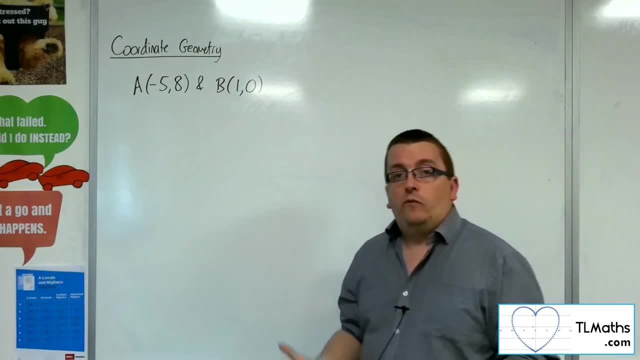 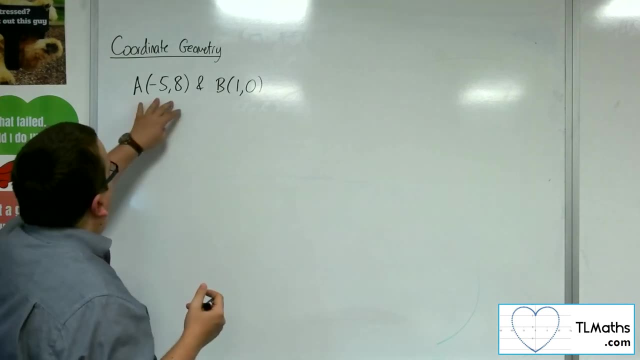 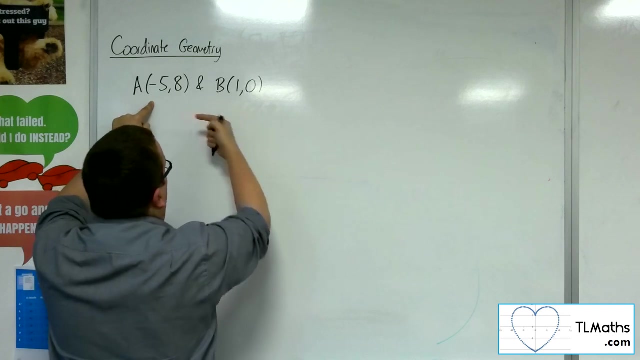 So drawing a little diagram or a little sketch of what's going on is really useful in these circumstances. So let's try and do that here Now. A at minus 5, 8 is over to the left and above B, because minus 5 is to the left of the 1 and 8 is above the 0. 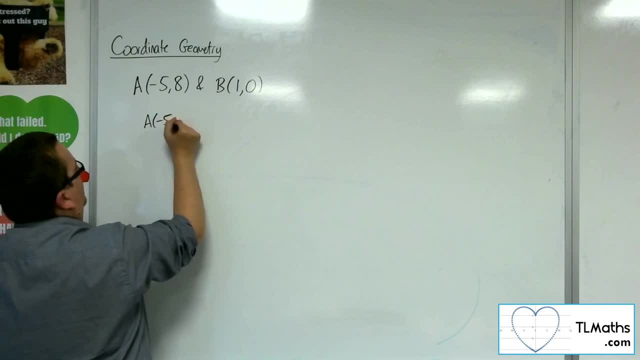 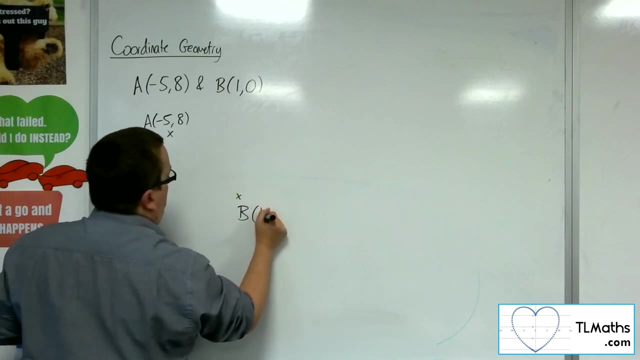 So if I put A over here minus 5,, 8, and so B would be somewhere to the right, a little bit further down, maybe somewhere here. So there's B at 1, 0.. You know, your diagram doesn't need to be perfect. 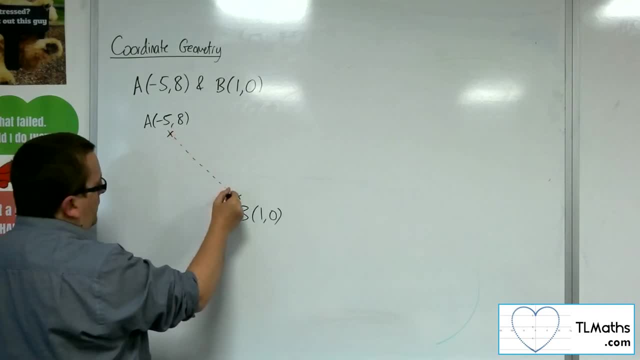 And I want to find that length And I'm going to call that length D. So I said that this utilises Pythagoras' theorem, Because what I can do is I can draw in a right-angled triangle where D is the hypotenuse. 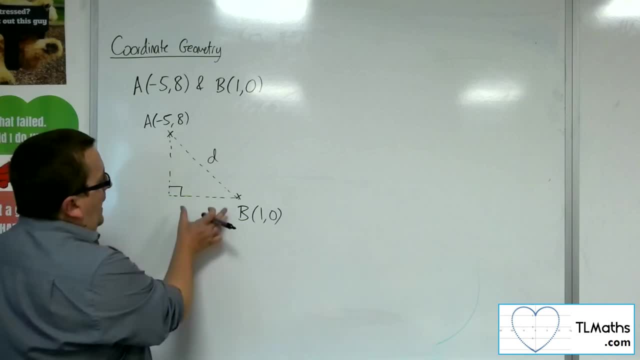 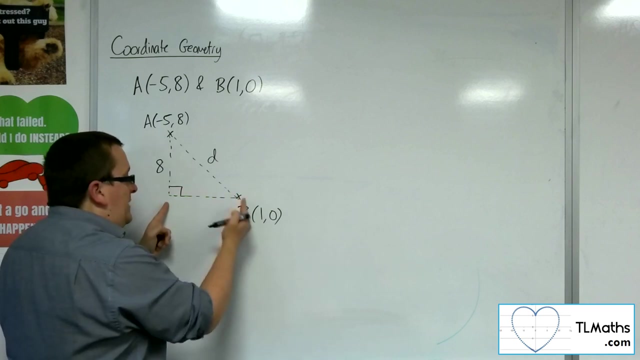 And this then leaves me to try and find the height and base of this triangle. So the height is going from 8 down to 0., So that would be of length 8. So 8, take away 0. And then for the x, for the base, we've got 1 to minus 5.. 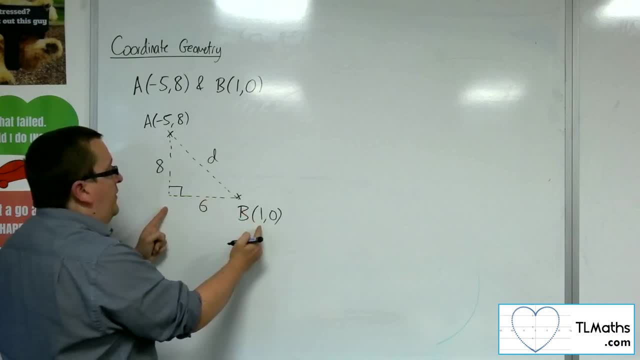 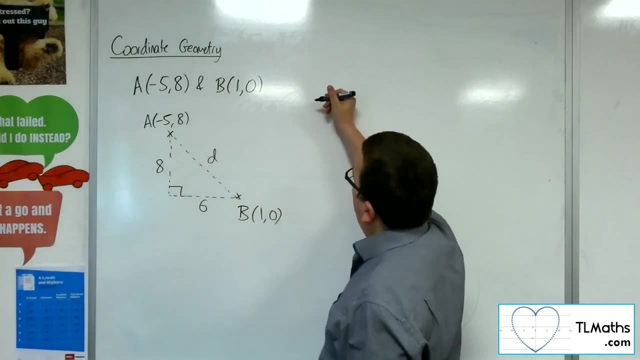 So that would be 6.. So that's 1, take away minus 5, which gets me to the 6.. So now I can use Pythagoras' theorem, which would say that D squared is equal to 8 squared plus 6 squared. 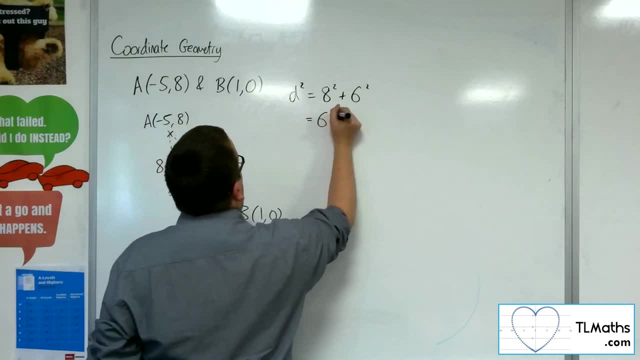 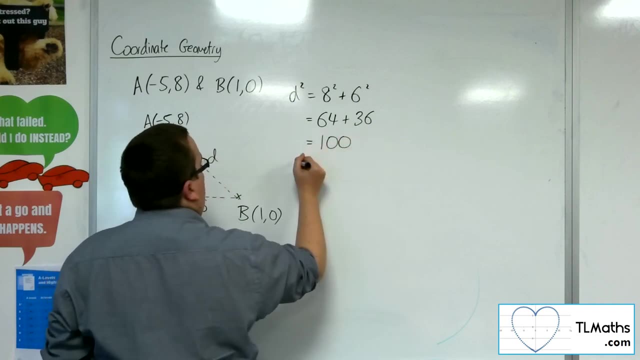 Now, 8 squared is 64. And 6 squared is 36.. And 6 squared is 36.. So 64 and 36 make 100.. And so D must be the square root of 100, which is 10.. 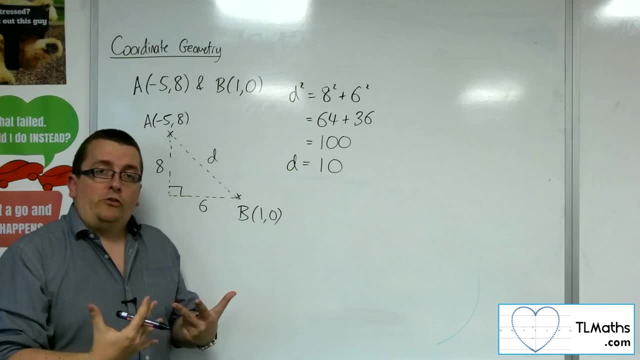 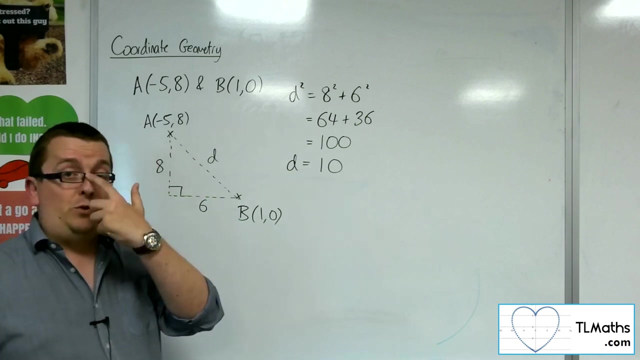 OK. So when you're square rooting here, you might be going: well, why isn't it plus or minus 10?? Well, we're talking about distance here. We can't really have negative distance. You can have a negative displacement, as we'll find later on in the course. 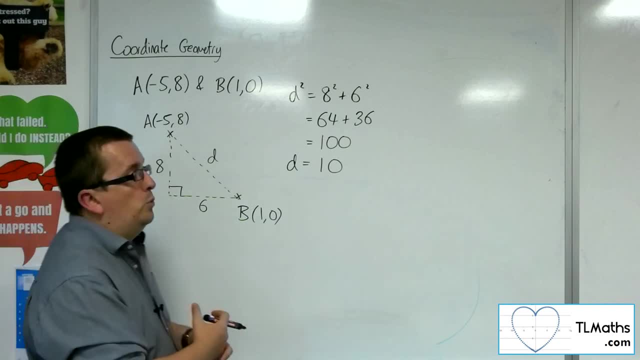 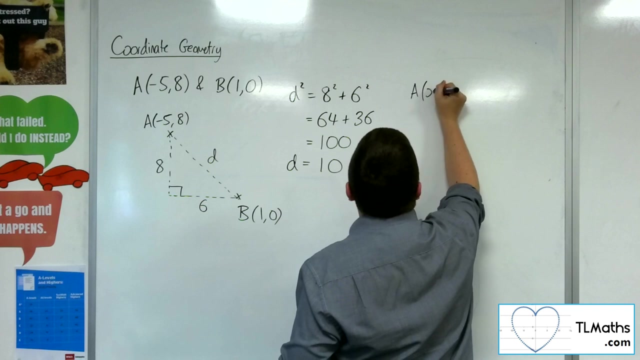 But distance is a positive quantity, OK, Much like area. OK, We don't talk about negative area. So if we're going to do this, generally, OK, and we have two coordinates, Let's say that A has the coordinates x1, y1. 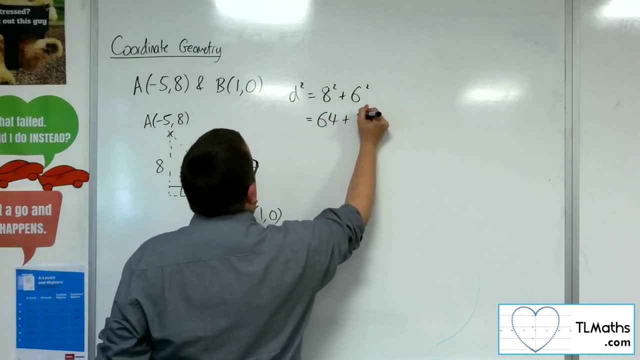 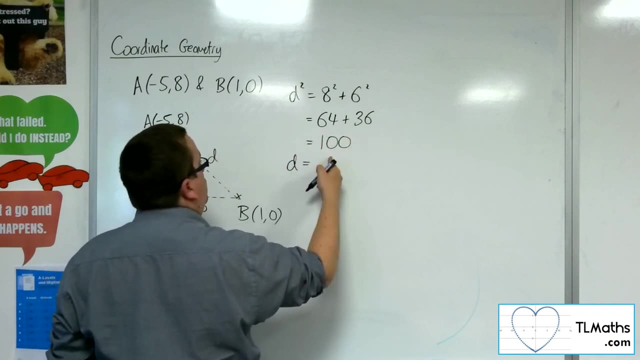 Now, 8 squared is 64.. And 6 squared is 36.. So 64 is equal to 8 squared plus 6 squared. So 64 and 36 make 100.. And so D must be the square root of 100, which is 10.. 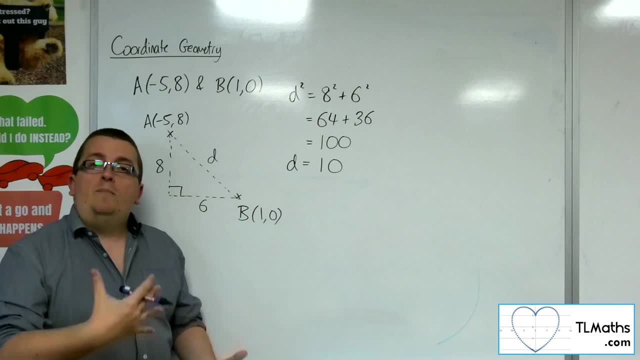 So when you're square rooting here, you might be going: well, why isn't it plus or minus 10?? Well, we're talking about distance here. We can't really have negative distance. You can have a negative displacement, as we'll find later on in the course. 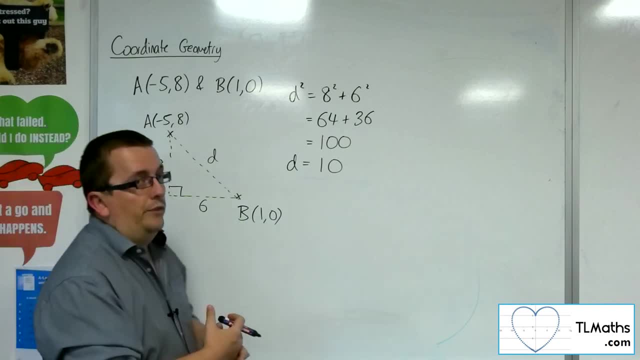 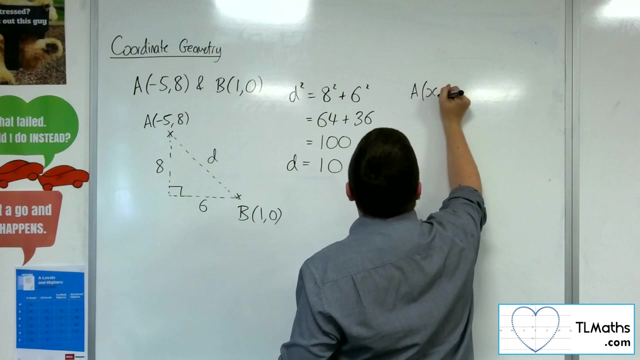 But distance is a positive quantity, OK, Much like area. OK, We don't talk about negative area. So if we're going to do this, generally, OK, and we have two coordinates, let's say that A has the coordinates x1, y1. 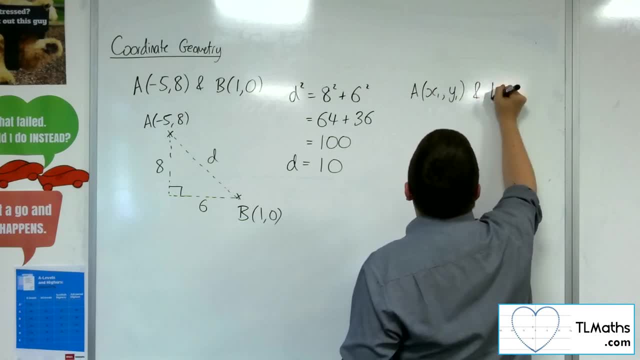 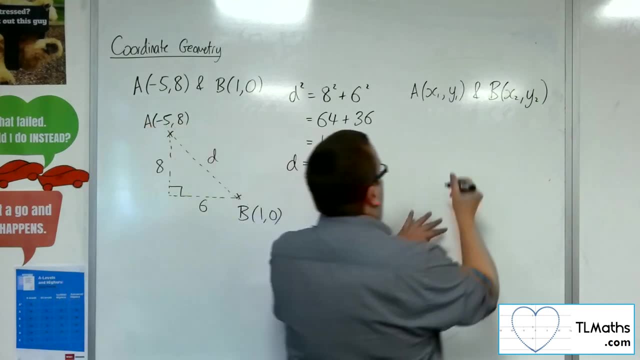 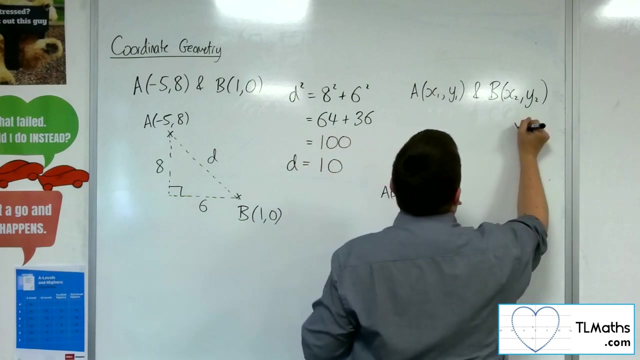 OK, It has its x and y coordinate And B has the coordinates x2, y2.. OK, Let's have another diagram. Here's A at x1, y2. Y1. And here's B at x2, y2.. 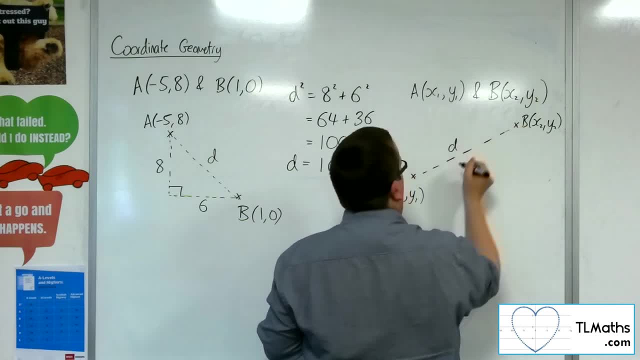 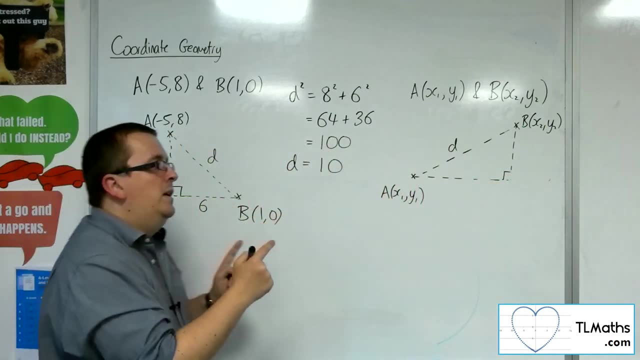 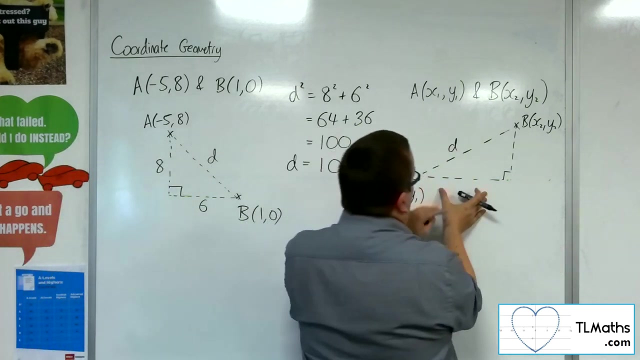 OK, And I want to find that distance. I can draw a right angle triangle, much like I did for the example. OK, And now I want to represent the height and base of that triangle using the algebra that we have. So the base of the triangle is looking at from x1 to x2.. 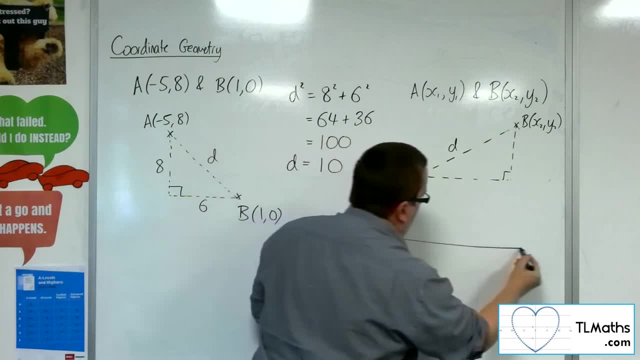 OK, Now, if you think of this as like an x-axis, and this was at I don't know 5, and this was at 11.. OK, How do I work out that distance? Well, I do 11. take away 5,, don't I? 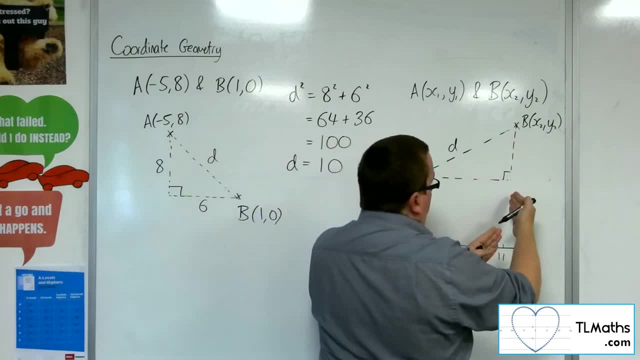 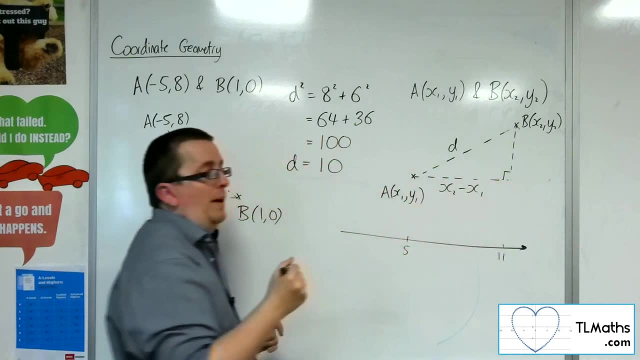 OK, Which is 6.. And so I'm doing x2, take away x1.. So this is x2 take away x1.. That's the length of the base of that right angle triangle. In a similar way, the height of the triangle is y2 to y1. 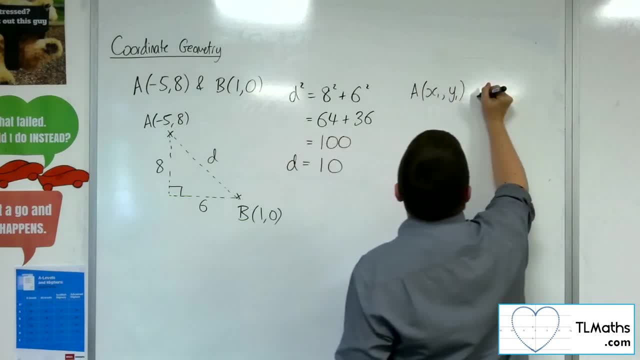 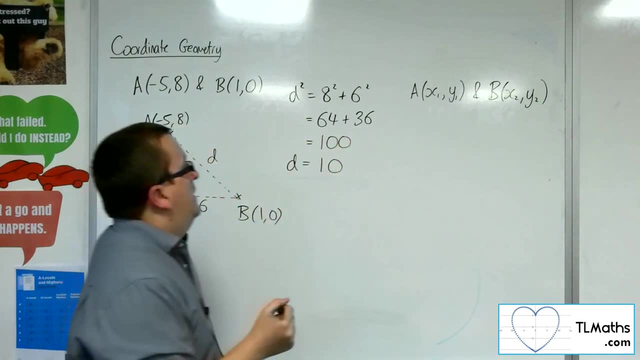 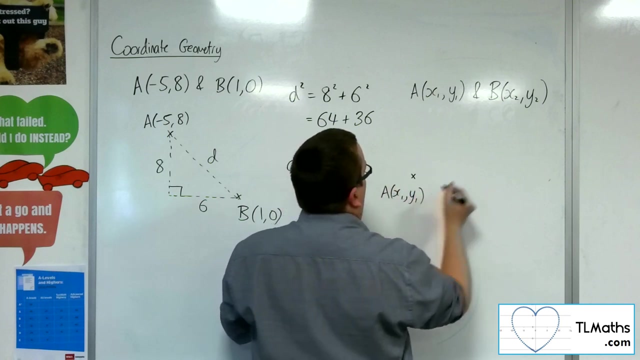 OK, It has its x and y coordinate And B has the coordinates x2, y2.. OK, Let's have another diagram. Here's A. Here's A at x1, y1.. And here's B at x2, y2.. 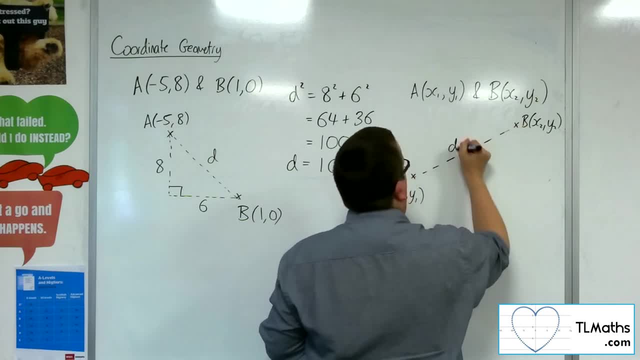 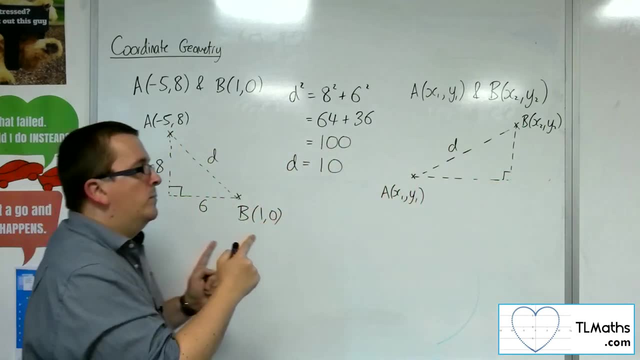 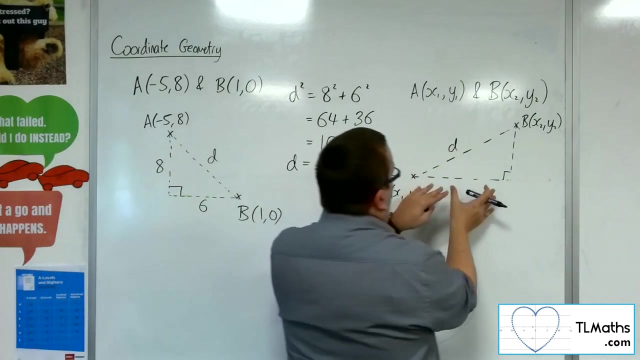 OK, And I want to find that distance. I can draw a right angle triangle, much like I did for the example. OK, And now I want to represent the height and base of that triangle using the algebra that we have. So the base of the triangle is this: 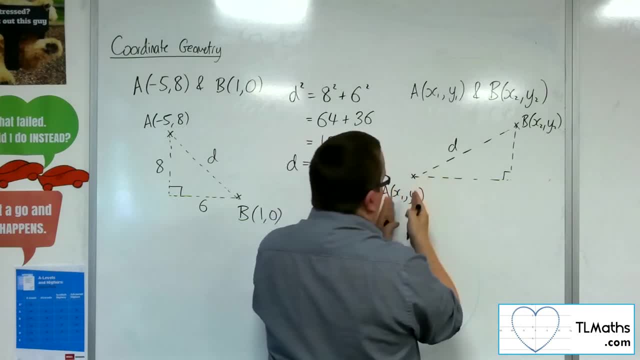 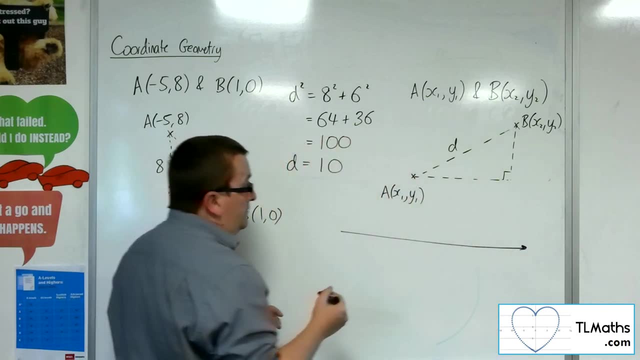 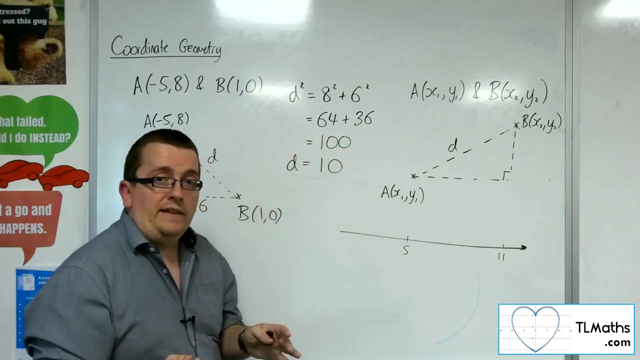 The triangle is looking at from x1 to x2.. OK, Now, if you think of this as like an x-axis, and this was at I don't know 5, and this was at 11.. OK, How do I work out that distance? 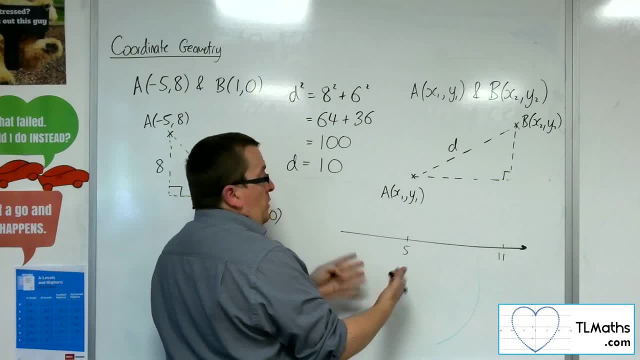 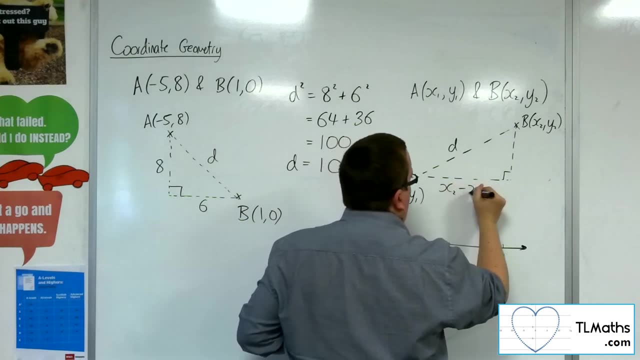 Well, I do 11, take away 5,, don't I? OK, Which is 6.. And so I'm doing x2, take away x1.. So this is x2, take away x1.. That's the length of the base of that right angle triangle. 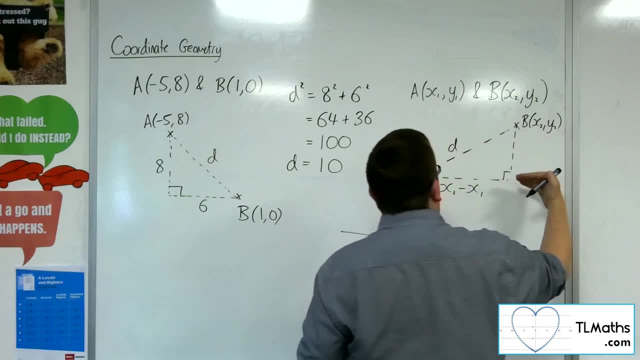 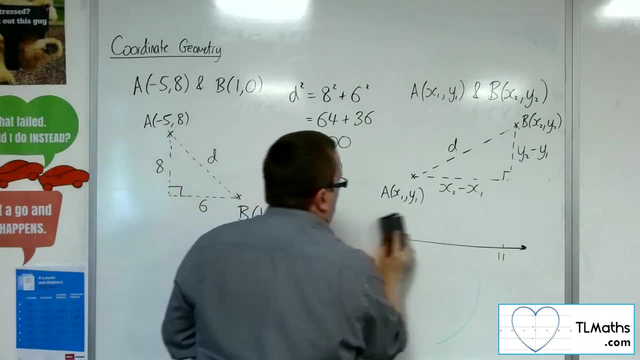 In a similar way, the height of the triangle is y2 to y1.. So y2, take away y1 in much the same way. So what we can now do, using Pythagoras, is say that d squared is equal to the base squared. 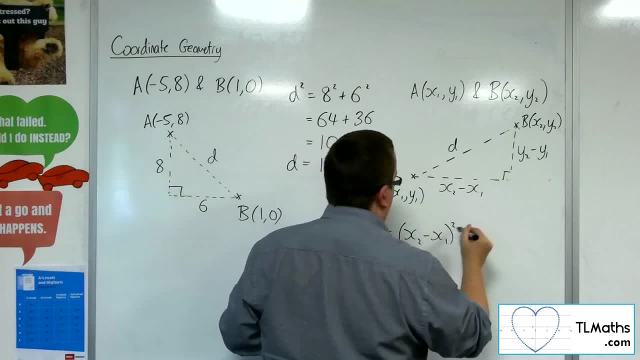 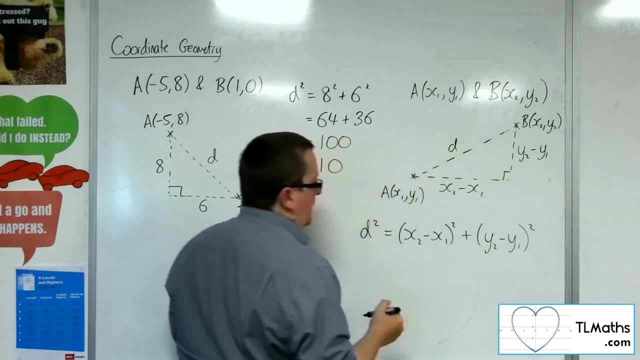 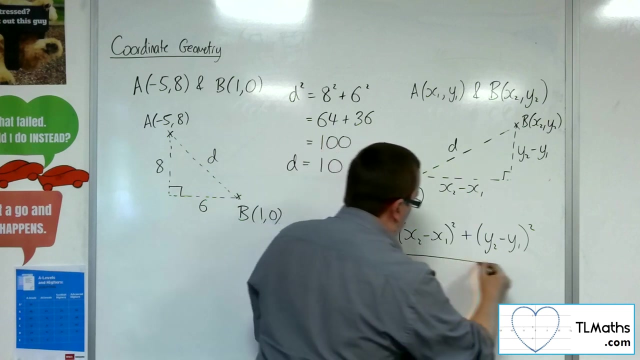 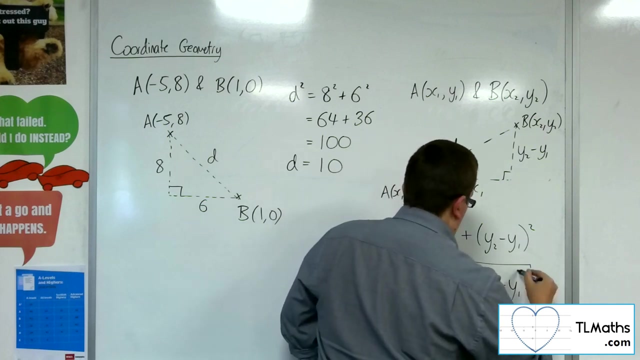 So x2 minus x1 squared, Plus the height of the triangle squared, y2 minus y1 squared, And so a general formula for the distance between two coordinates will be the square root of x2 minus x1 squared, plus y2 minus y1 squared. 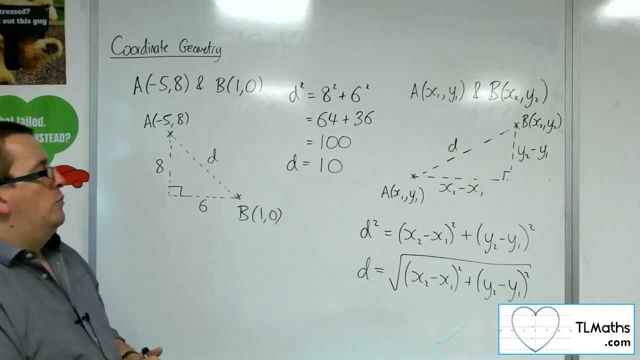 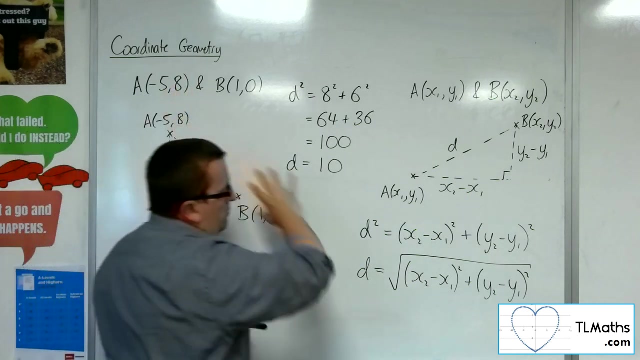 OK, So that would be the general formula that we can utilise. Now, personally, The way that I would go about this if I was given the two coordinates like that, I don't generically go. well, generally go straight to the formula. 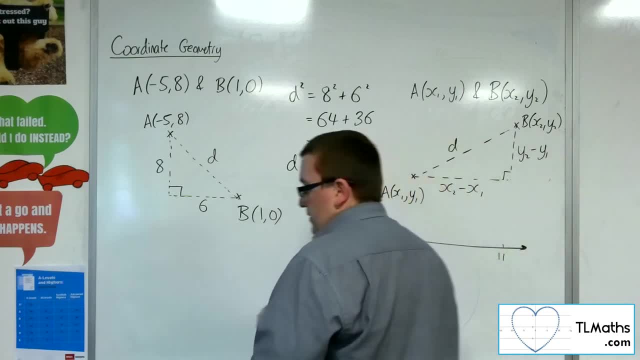 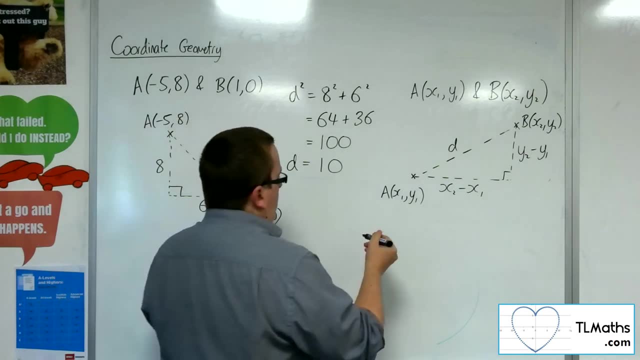 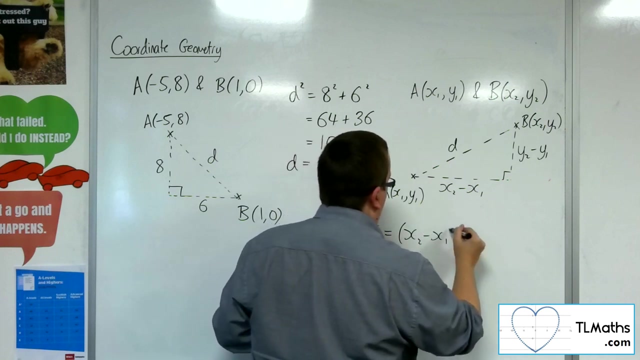 So y2. take away y1 in much the same way. So what we can now do using Pythagoras is say that d squared is equal to the base squared. so x2 minus x1 squared plus the height of the triangle squared. y2 minus y1 squared. 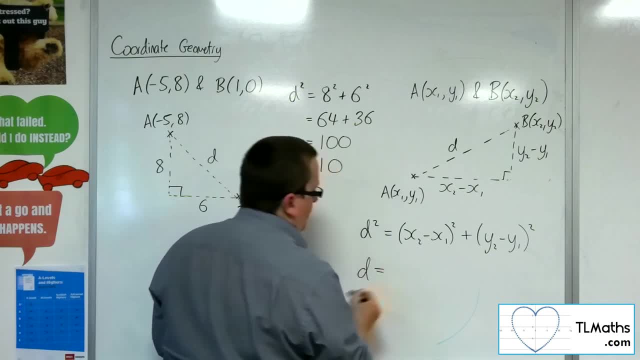 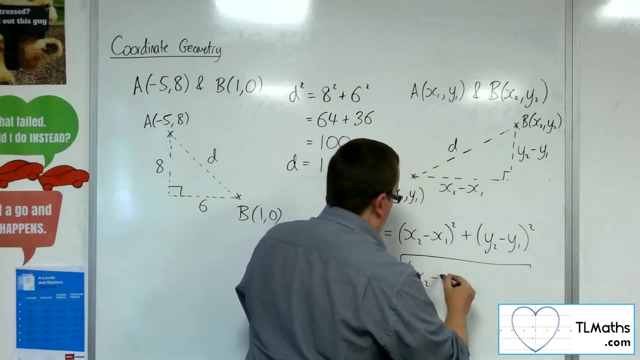 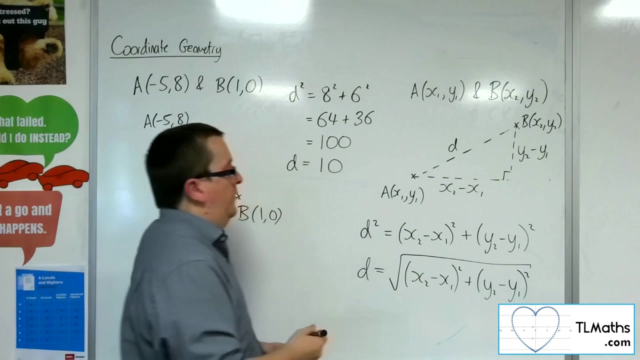 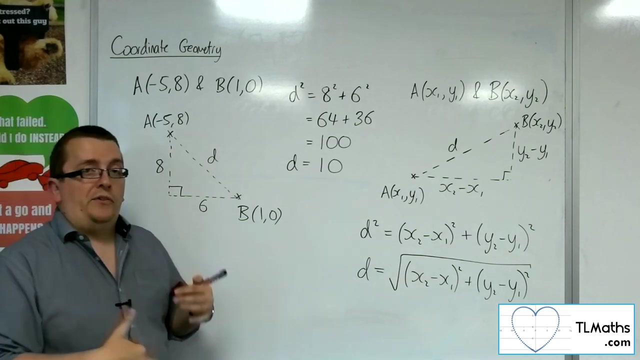 And so a general formula for the distance between two coordinates will be the square root of x2 minus x1 squared plus y2 minus y1 squared. OK, So that would be the general formula that we can utilise. Now, personally, the way that I would go about this: 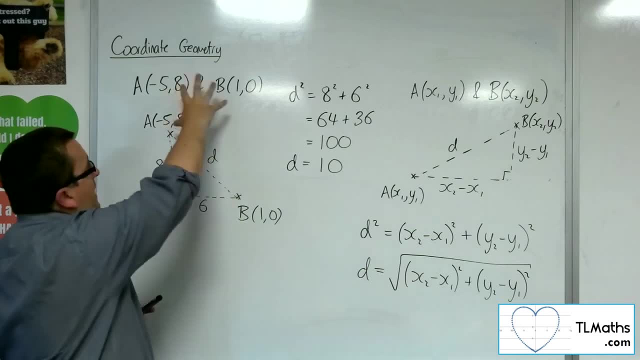 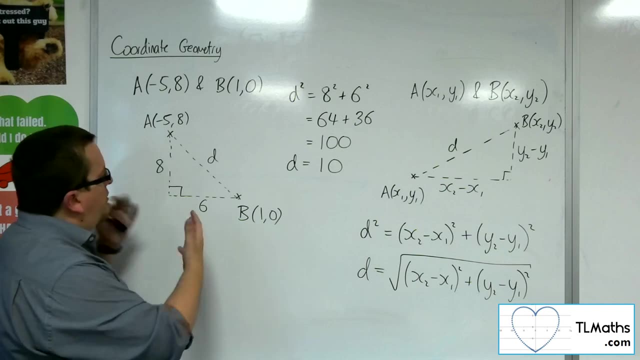 if I was given the two coordinates like that? I don't generically- well generally go straight to the formula. That's not usually how my brain works. I usually like to draw a little diagram so I can visualise where the coordinates are. 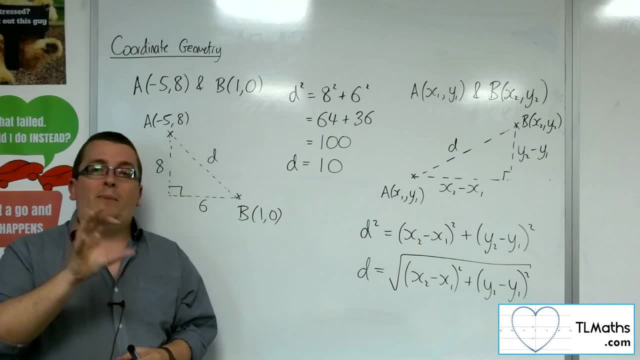 draw a triangle and then think about the base and height and use Pythagoras that way. If you want to go on and utilise and memorise the formula and use that, then that's fine. That will get you your answer. 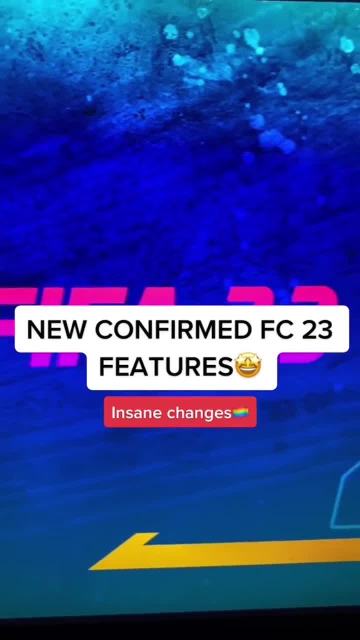 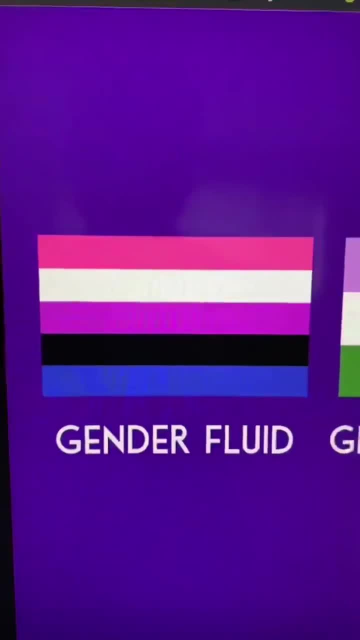 Three new features EA have confirmed they're adding to next year's EA Sports episode. The stuff is that there will be a new full LGBT team that you can play with in kick-off, That in career mode you'll have four choices from gender fluid. 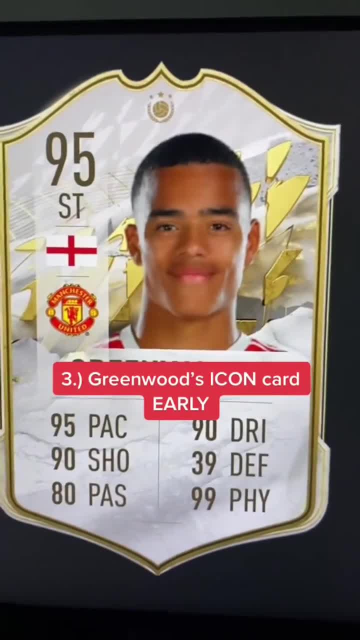 gender, queer and the other two to choose from. Since Greenwood can't play football anymore, they're officially going to retire him and give him his icon card. 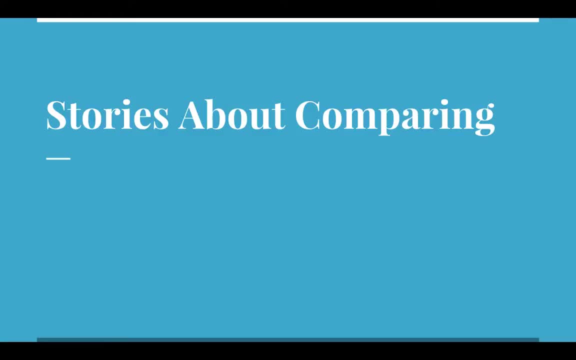 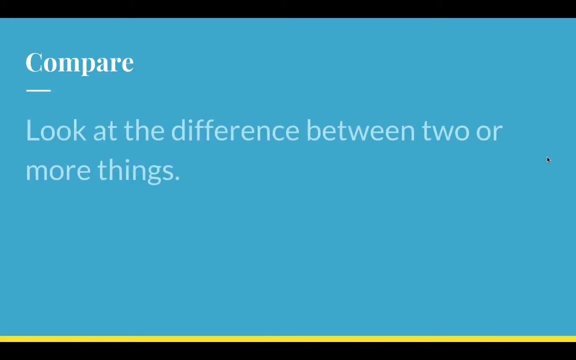 In this video we're going to learn about stories about comparing. So we'll look at story problems that compare two different quantities or numbers. First we need to look at what the word compare means. So compare means looking at the difference between two or more things. So we're seeing, maybe, what's the same or 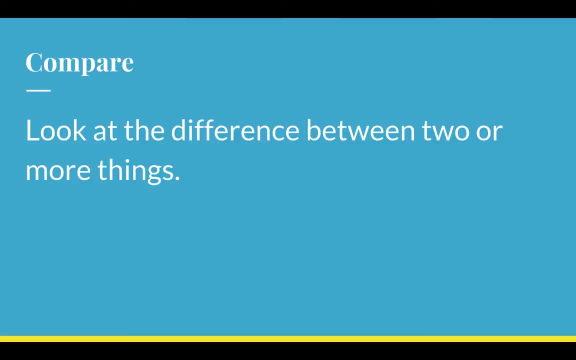 what's different and, specifically, what's different about the numbers. Some keywords that we'll be looking for in comparing problems are how many more and how many fewer. Usually, when you see these phrases in story problems and it's asking you to find how many more or how many fewer, you can use the comparing strategy to help.